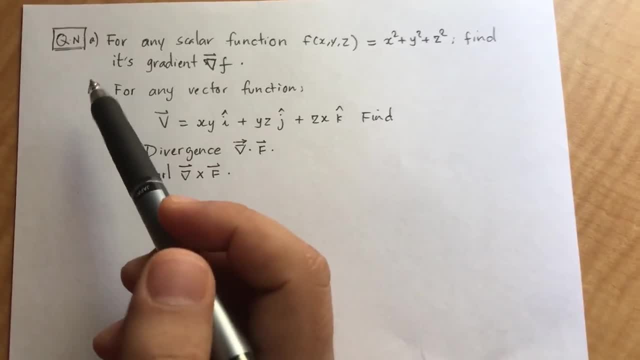 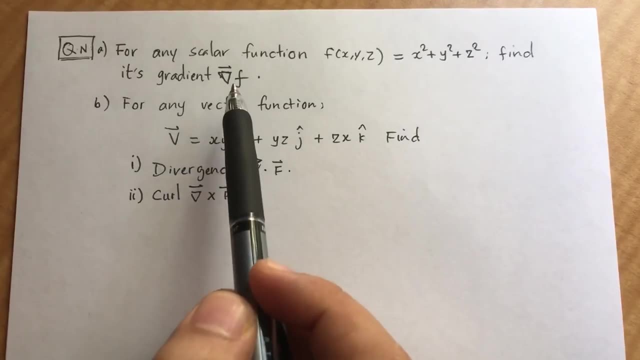 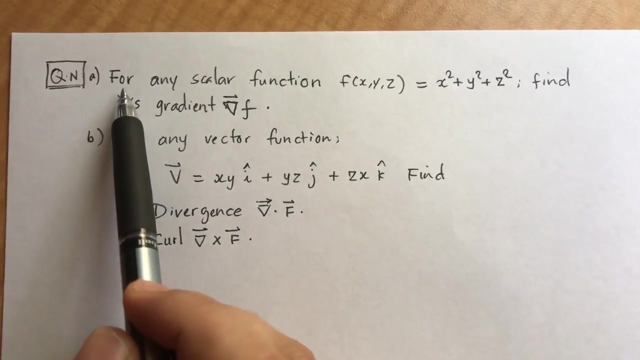 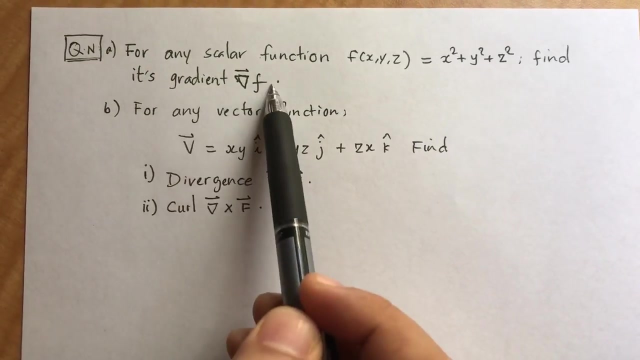 hi everyone. today I am back for my second video, so this will be a simple problem related to divergence, crawl and gradient of a given function. so in the first question I have here a function depending on X, Y and Z, and then I have to find the gradient of this one, whereas in the second question I have another. 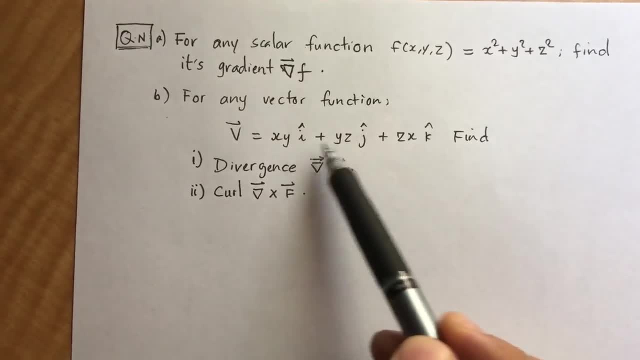 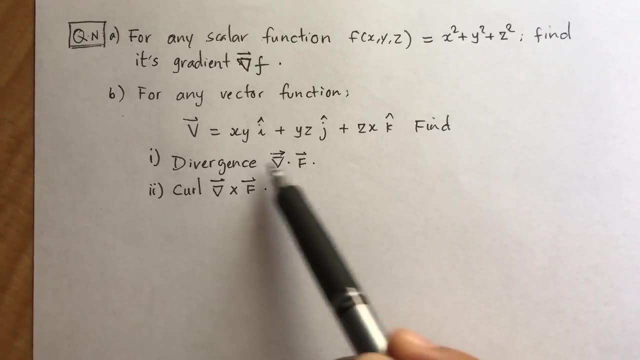 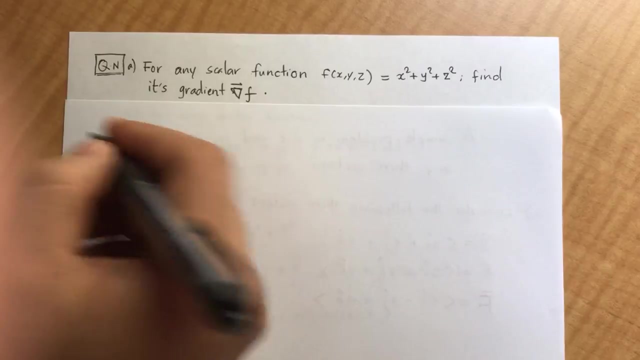 function vector function X, Y I hat plus Y Z, Z hat plus Z X K hat. and then I am told to find the divergence and the call of this one. all right, let's start with the first problem. so it wants us to calculate the gradient of given function. 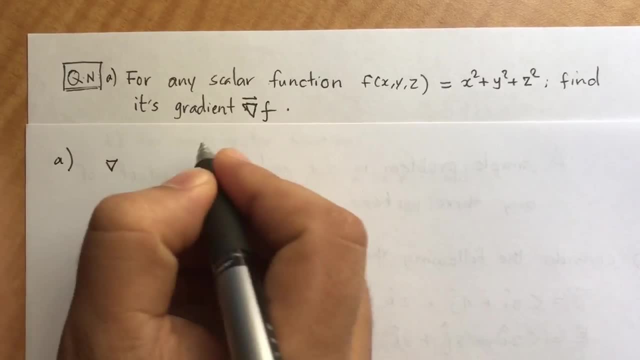 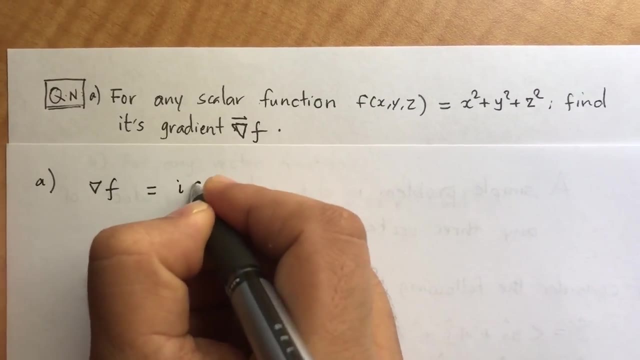 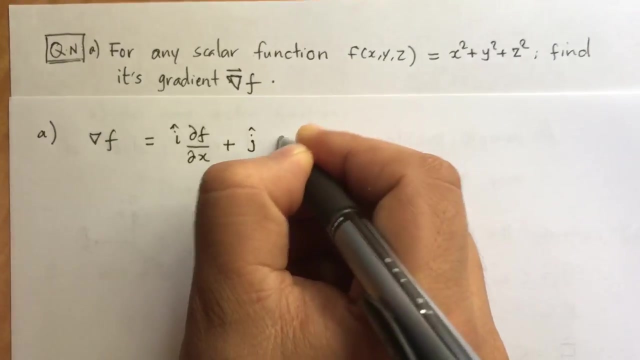 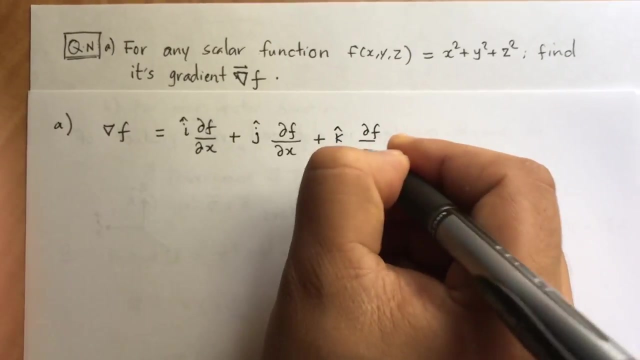 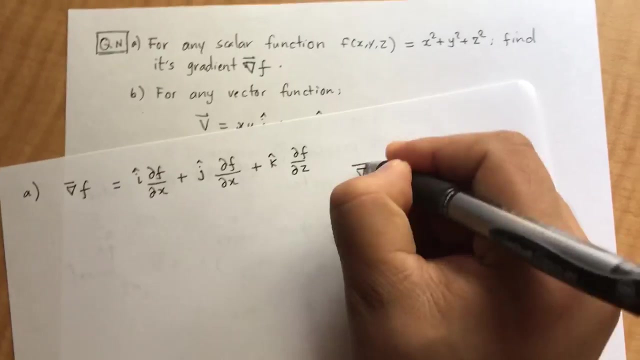 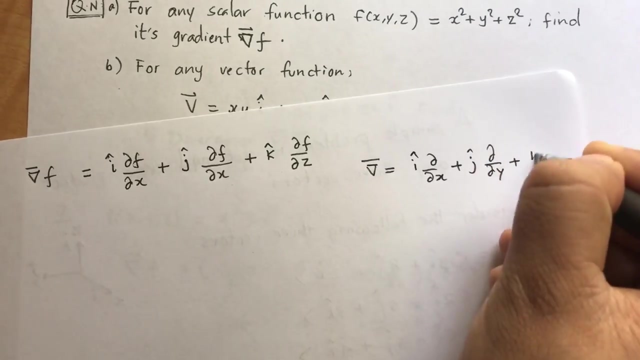 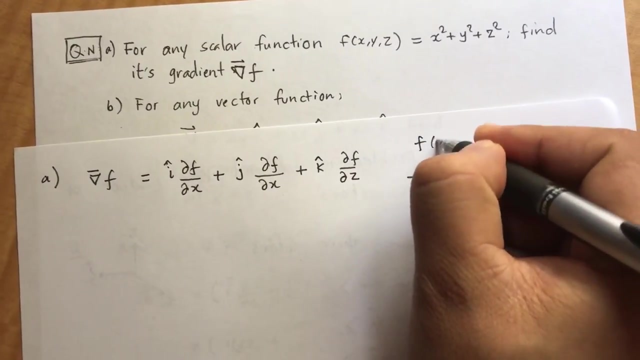 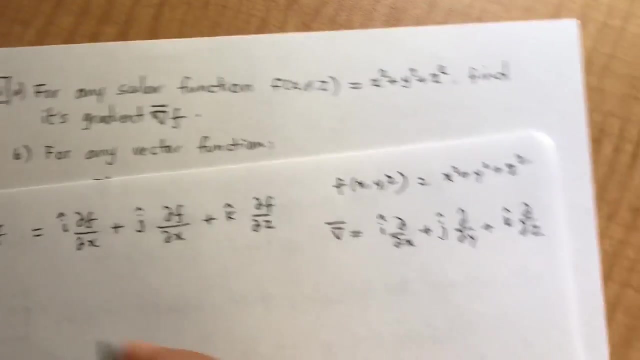 that is, it wants us to calculate the, that F, which is actually I df by DX plus, say, df by DX plus K df by DC. so this is because this is because we have: Delta is equal to I d by DX plus C d by dy plus. and then we also have F, X, Y, Z is equal to X square plus Y square plus Z square. 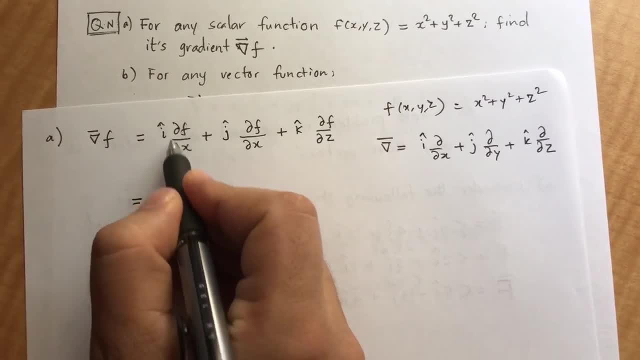 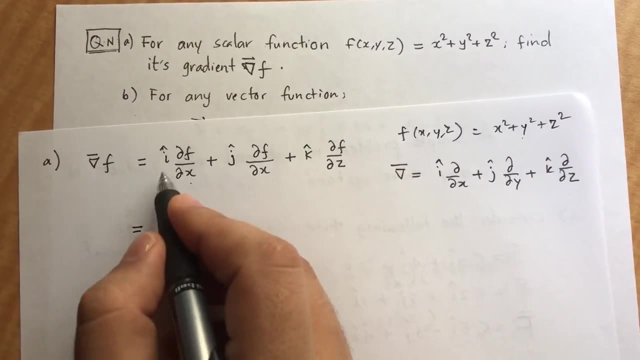 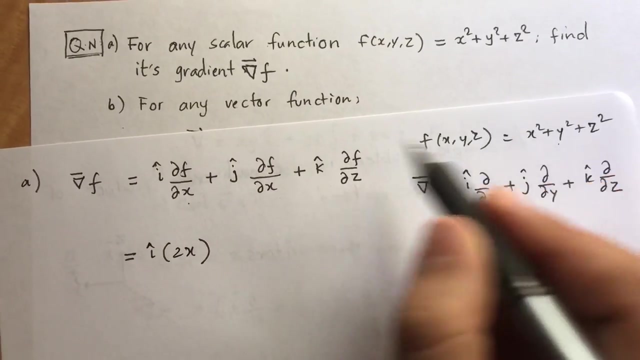 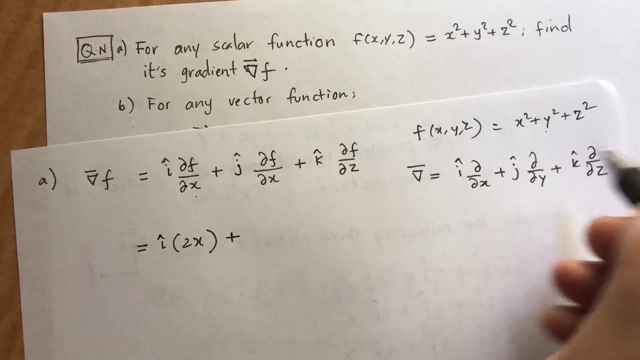 now, when I'm taking, the partial derivative of F with respect to X, Y and Z will be considered constant, so the first term over here will give me twice X, because the derivative of X squared with respect to X is twice X, whereas this two quantities won't be giving me anything. similarly, over here I'll be getting and. 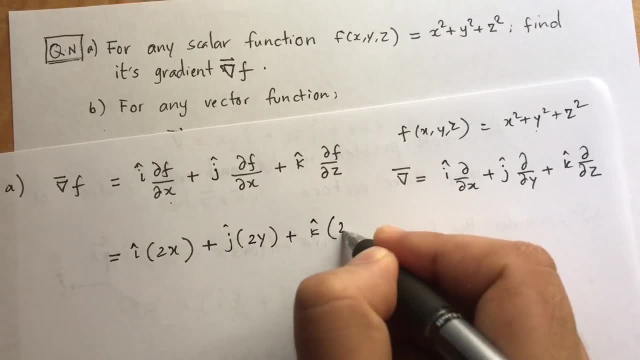 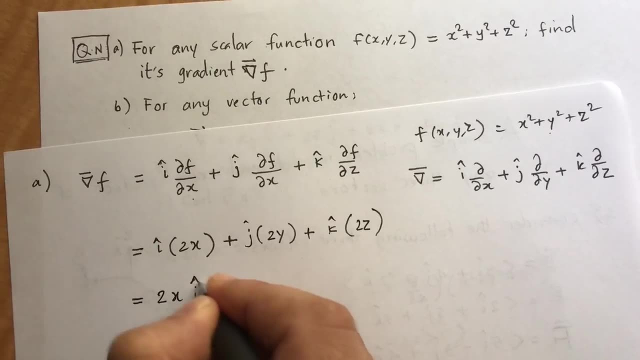 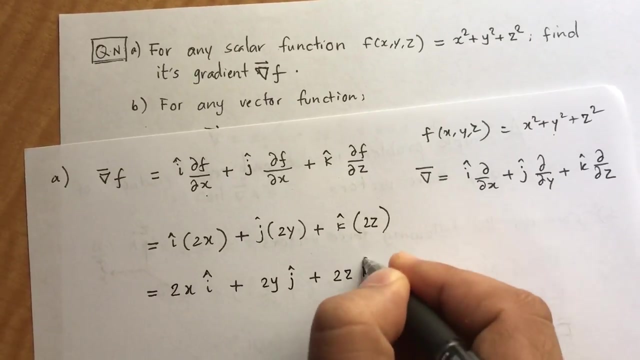 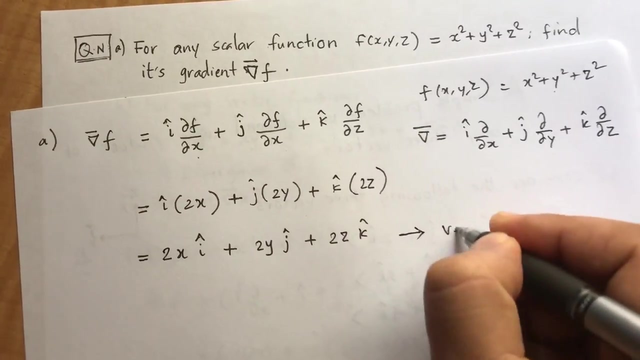 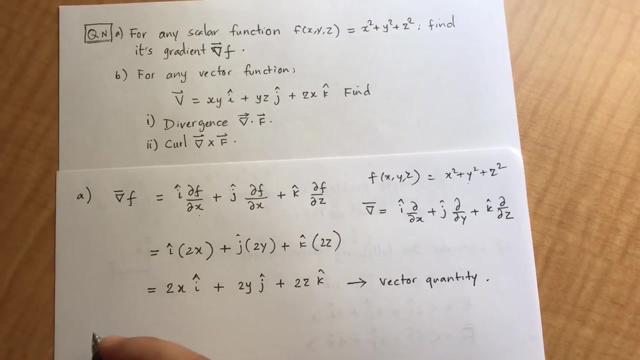 then finally over here I'll be getting twice Z. so this will be finally twice X I hat, plus twice Y, Z hat, plus twice Z k hat, and all of you can see. the gradient of any scalar function will give me a vector quantity. all right, guys, let's now go to second problem. so in 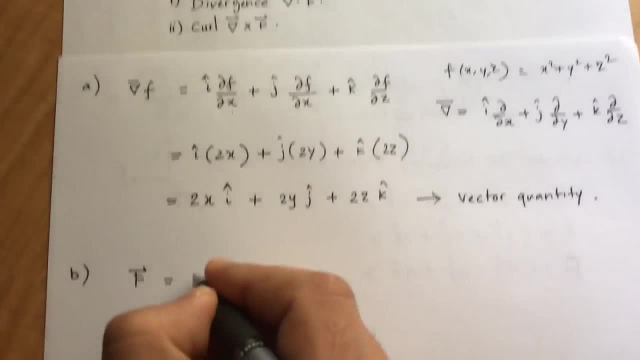 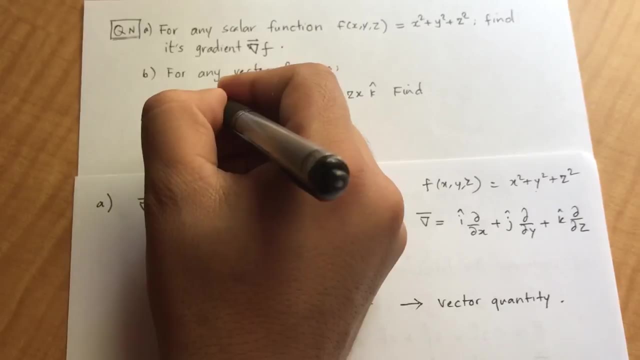 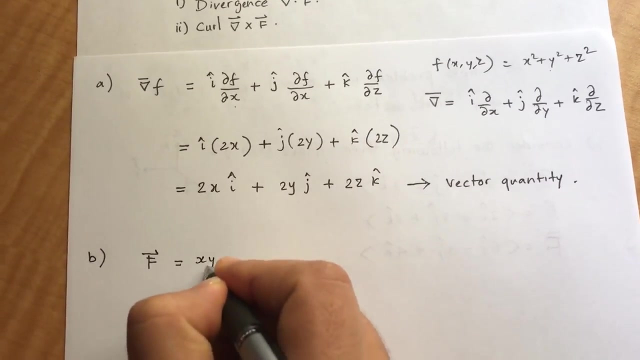 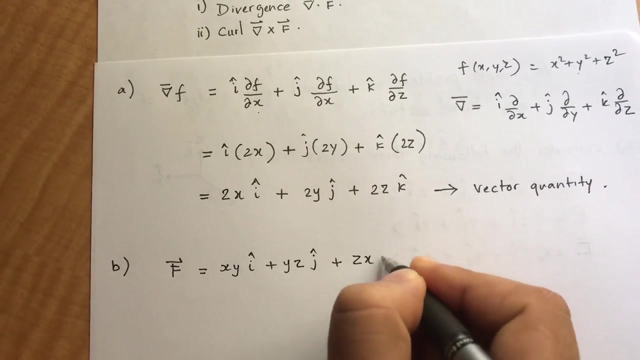 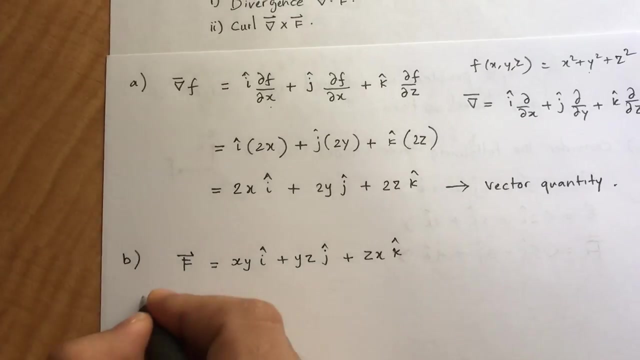 second problem: I have a vector function, F. actually it's denoted by V over here, but it's it's a typo. so this is: this is F. so F is actually equal to X, Y, I plus Y, Z, Z plus Z, X, k. now I'm told to calculate the divergence of this function in first question. so if I 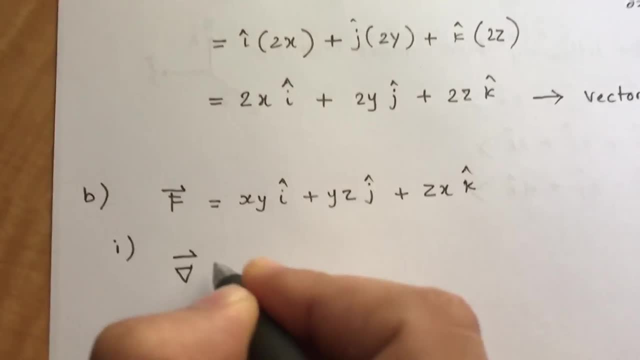 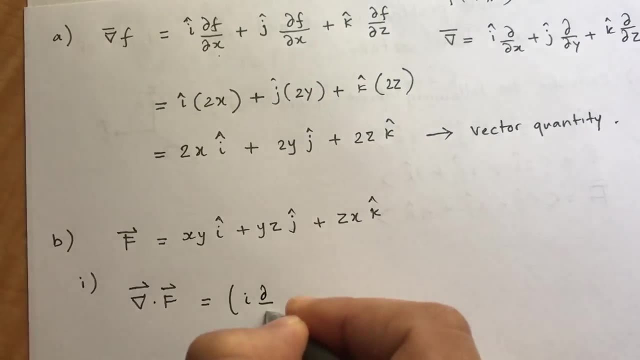 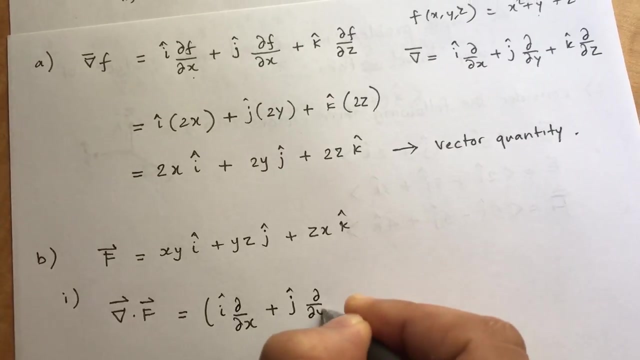 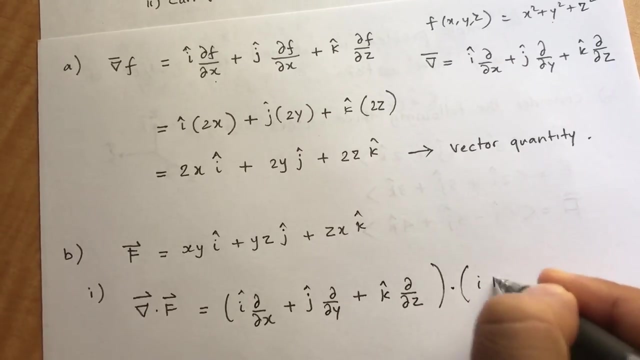 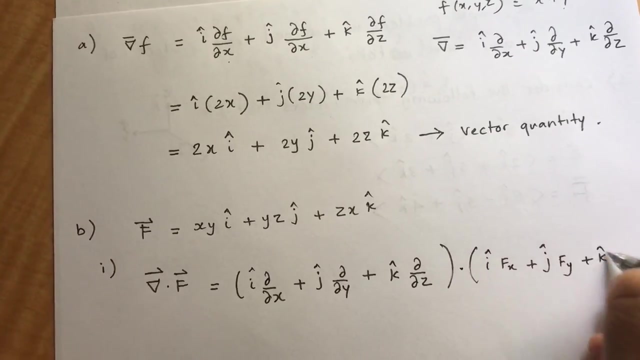 calculate its divergence. this will give me divided X, X plus Z, Y dot X, Y, X plus Y dot Z pressure I F, z dot. divided Y plus YouTube bar plus a mı gl ב� X plus bit by D, y plus K. divide easy, dotted with I, FX plus we see F, Y plus K, Z. so over here V, over here, wait, I'll combine them again with repetitions. so over here we have W, over here we will. 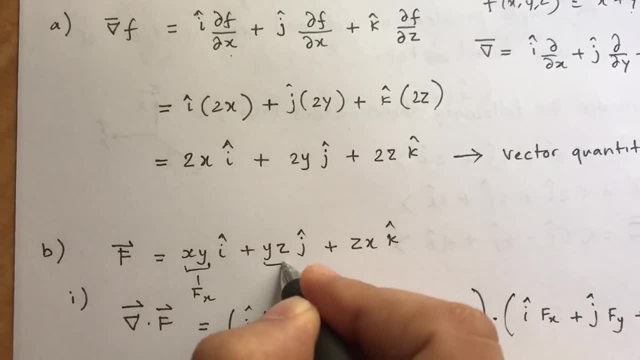 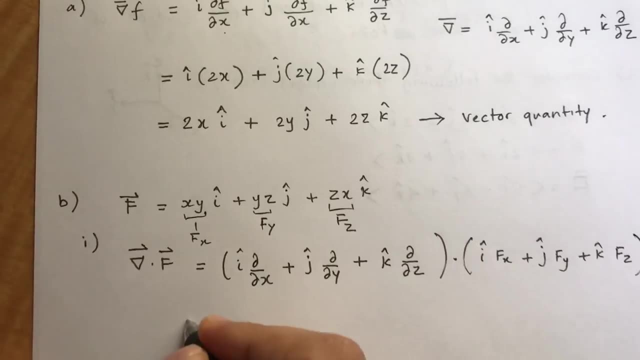 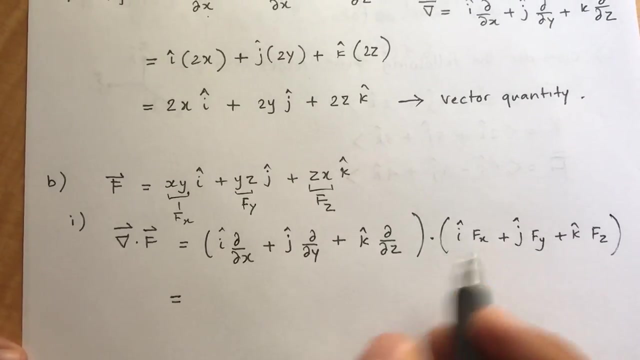 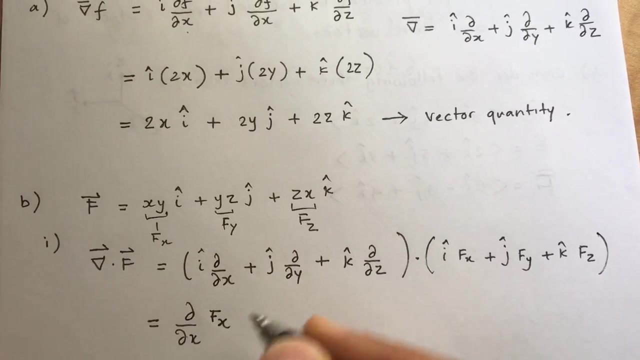 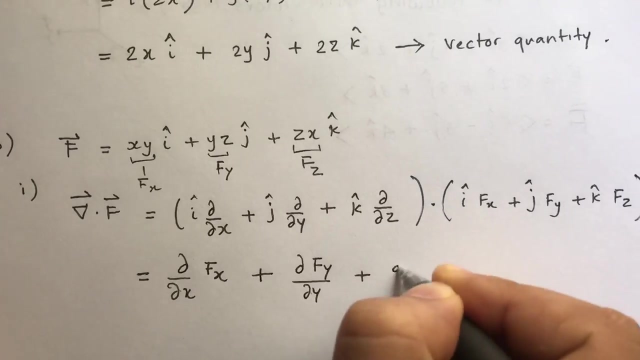 whatever this is, this is fx, this is fy, this is fz right? So if I proceed further, when I'm taking dot- product I have already mentioned in my previous video, so this will be like partial of fx with respect to x plus partial of fy with respect to y plus partial of fz with. 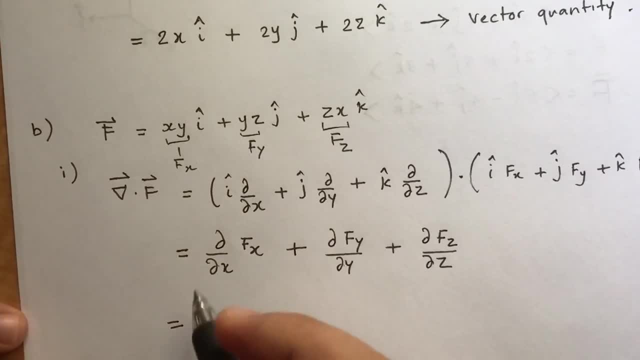 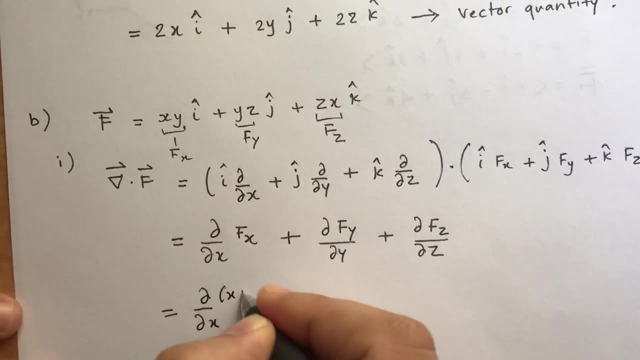 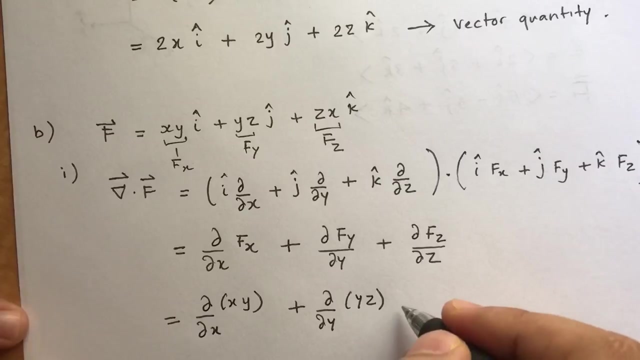 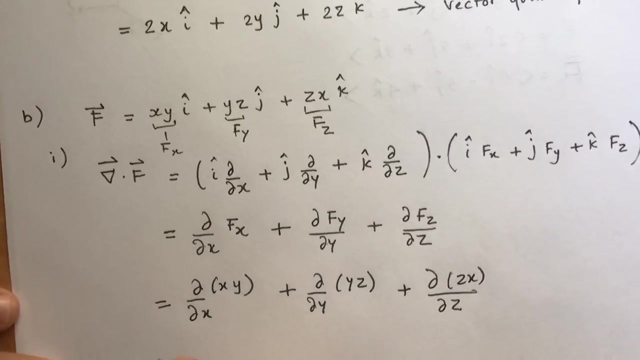 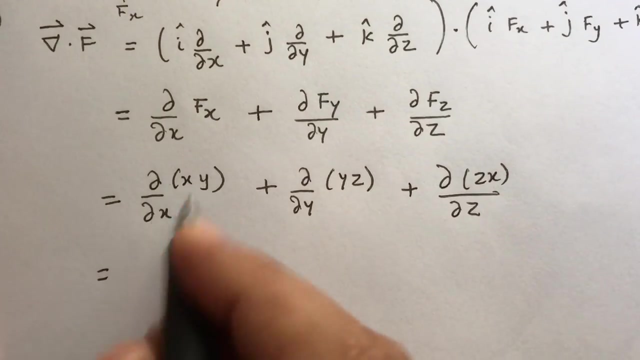 respect to z. So partial of xy with respect to x, plus partial of y with respect to z, yz with respect to y, plus partial of zx with respect to z, As I've already mentioned over here. so this particular quantity, y, is now considered constant. so it will come out, so it will give me 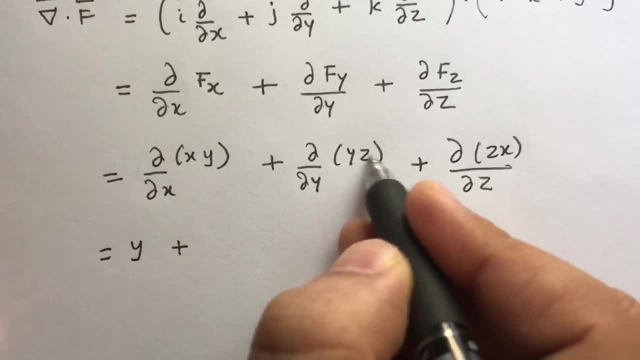 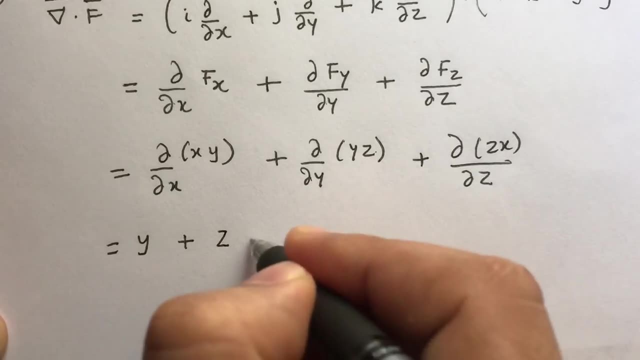 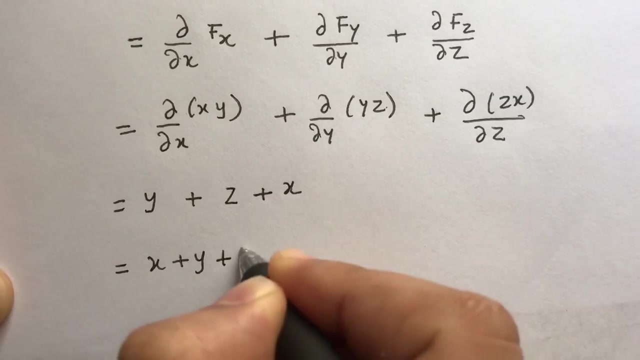 y over here, the quantity z will come out. so dy by dy will be again 1, that will give me z, and then over here I'll get x. So my final divergence will be x plus y plus z. You can clearly see over here: 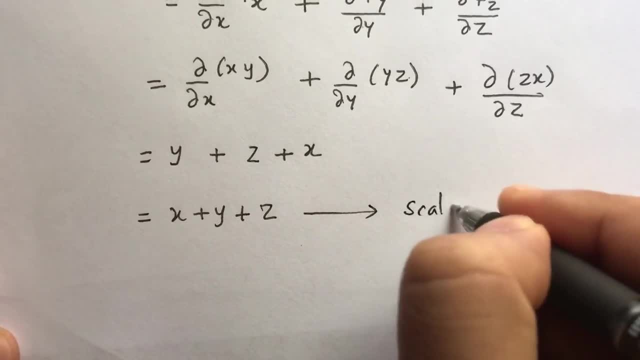 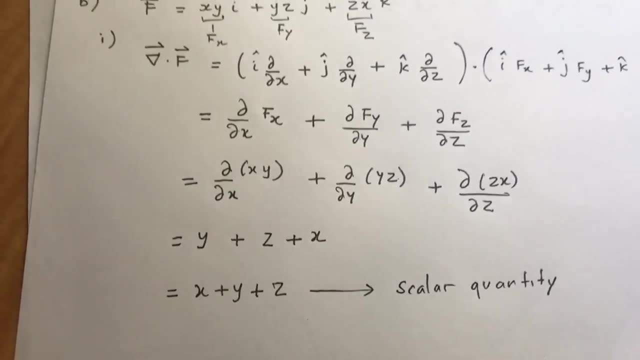 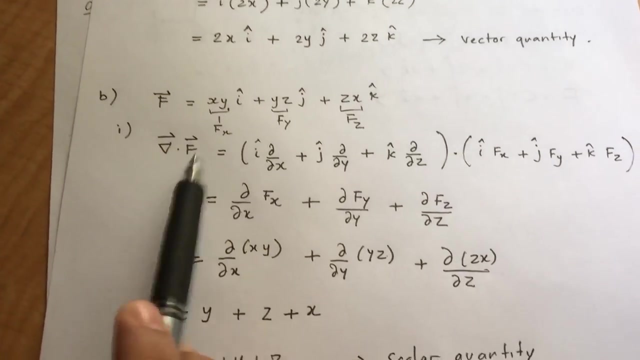 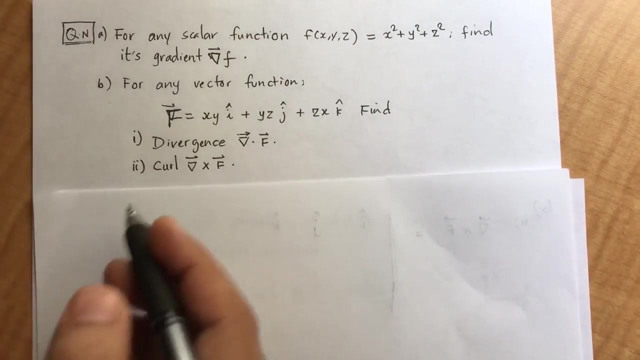 this is a scalar quantity. so that is perfectly in an agreement with our previous question in previous video. so if you do a dot product putting any two quantities, you should be getting a scalar quantity. that's why we call it scalar product. nice, we are finally back to our third problem. so over here in third problem we are: 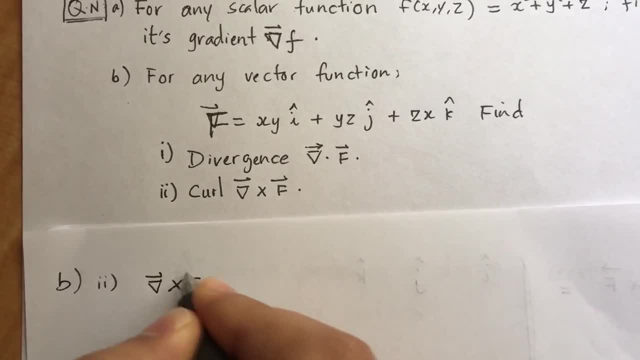 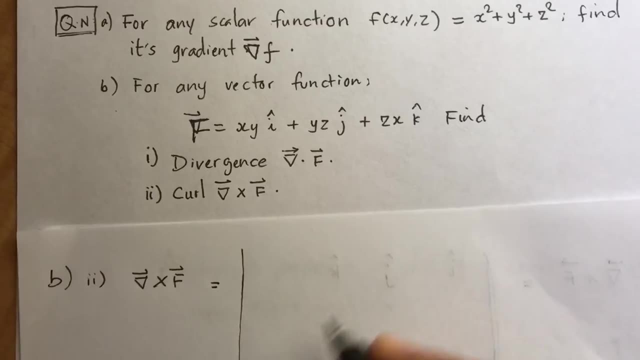 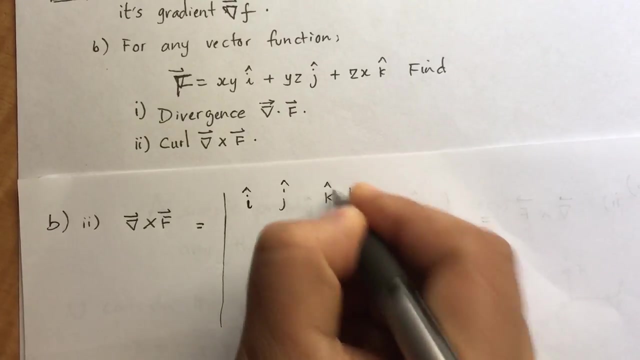 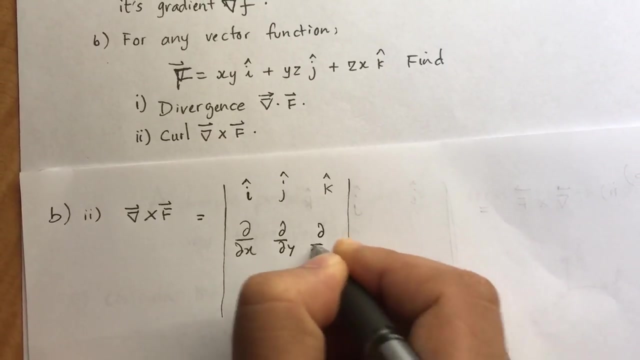 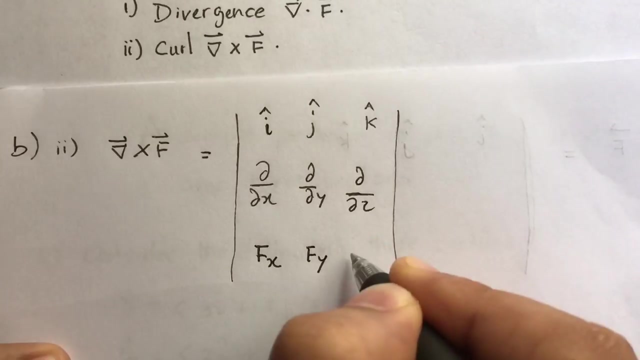 supposed to calculate the curl of given vector F. so if you actually review the definition of curl it can be actually written in determinant form. so it can be written like I say K, and then dy, dx, dy, dy, dy, dz, and then finally the vector is F, X component of vector, Y, component of vector and then Z, component of vector. 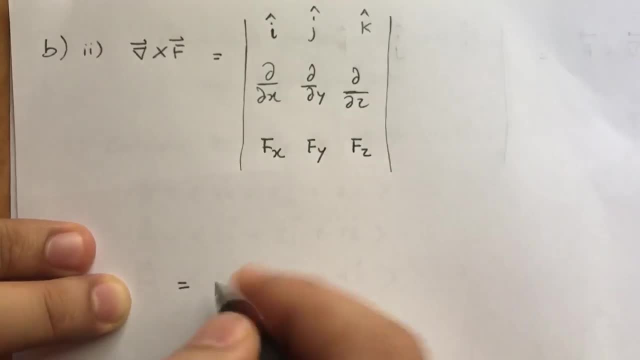 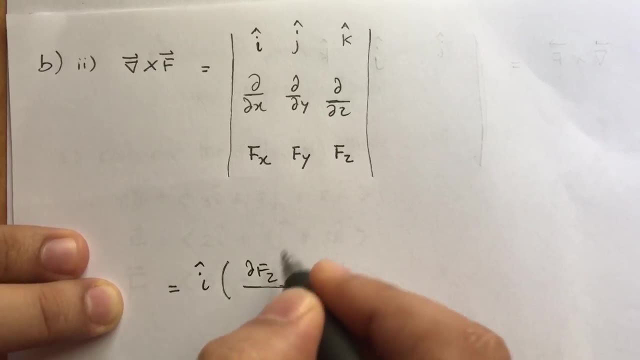 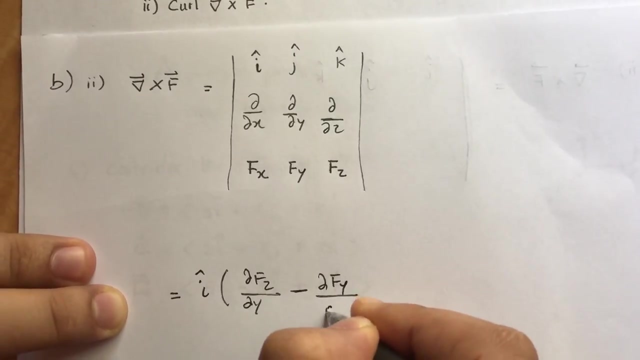 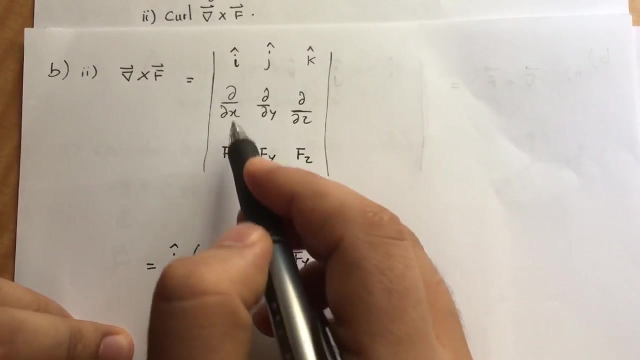 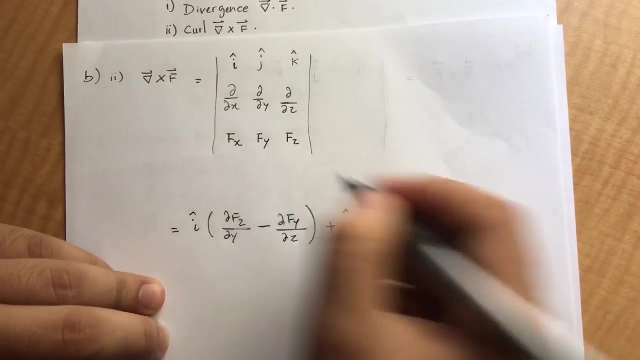 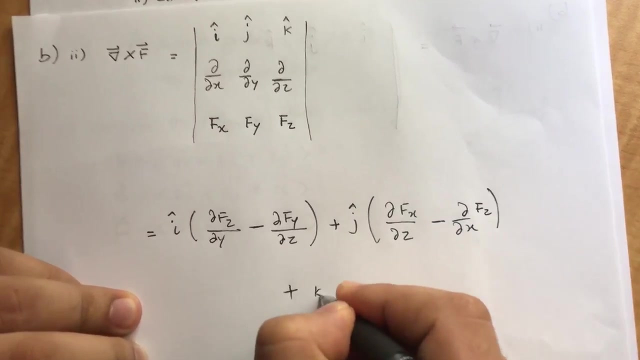 so if I expand this, I can actually expand this in such a way that the I component will be actually DL, see over dy minus df, y over DC plus, say component, will be so dx over DC minus divided X, Fz. and then finally, in the component of vector y, component x is minus DG or factor of y, which is the Dennis game, and then finally the capital English, and then I combine the otherstones and draw the matrix of expect, recognizes, and then finally the integral is their. 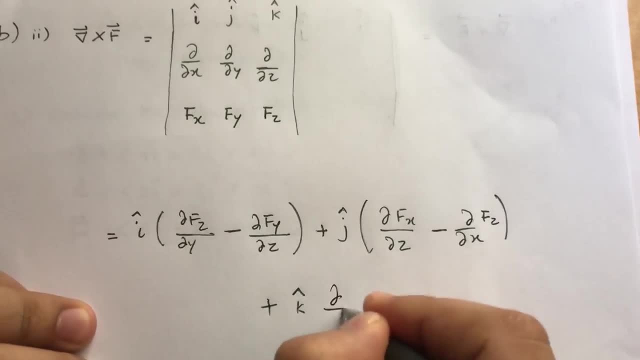 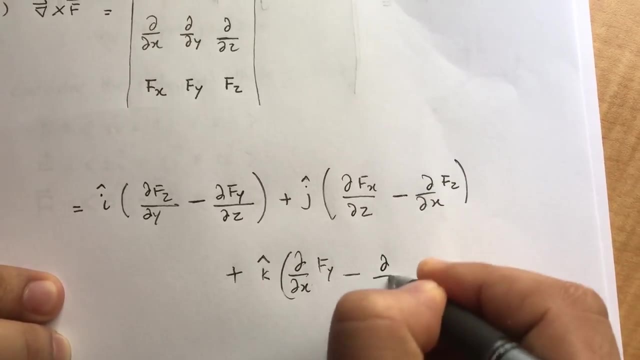 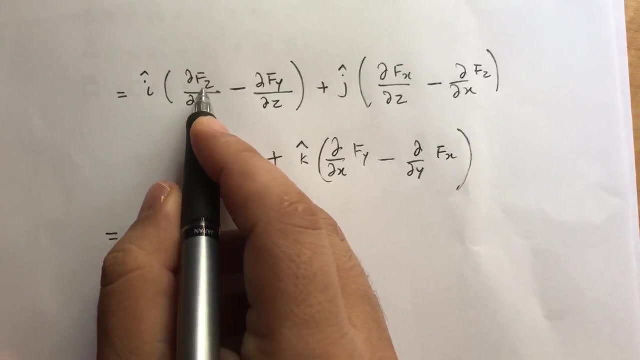 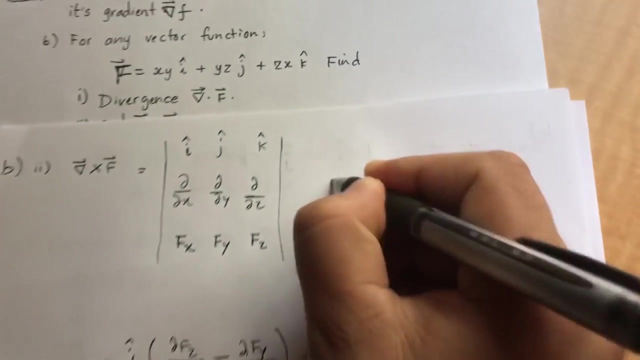 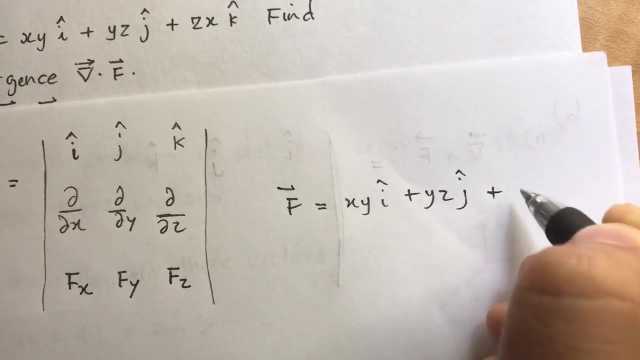 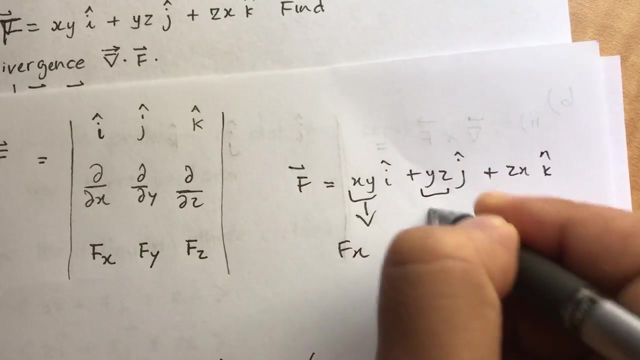 k component will be d by dx of Fy minus d by dy of Fx. all right, so now the partial of Fz with respect to dy. so we have this vector function: Fxy, i plus yz, z plus zx k. so this is my Fx, this is my Fy, and then this is my Fz. so if I go, 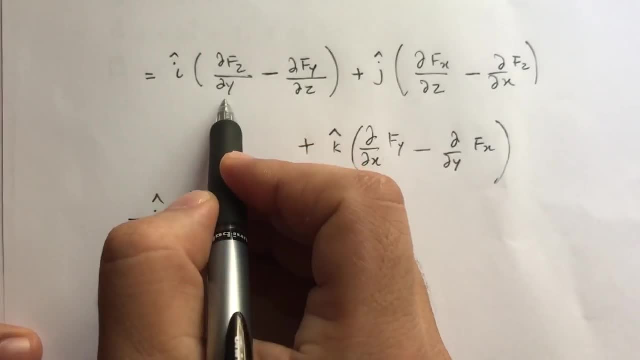 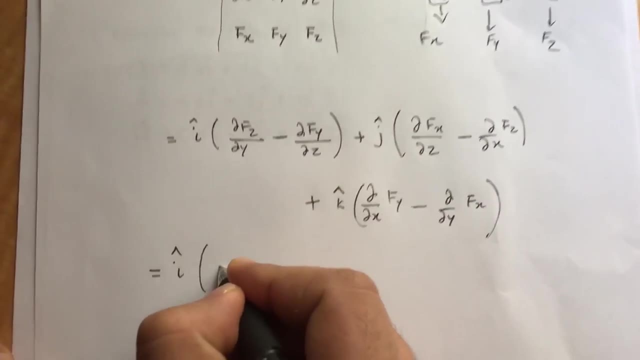 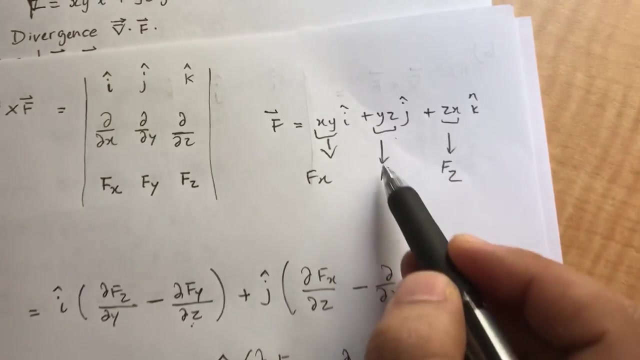 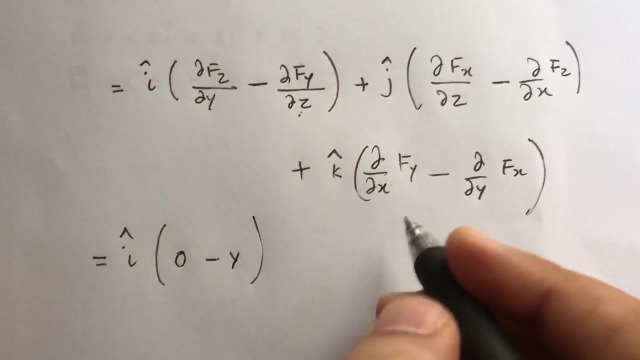 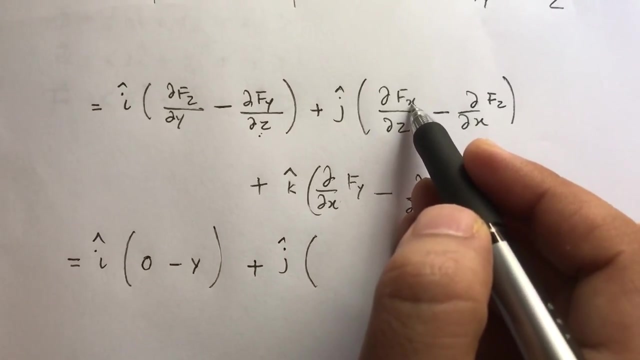 here, over here. d by dy of Fz. where is our Fz? it's over here. so Fz, this quantity is actually zero minus dFy over dz. so this quantity will actually give me dFy over dz. it will give me y right similarly over here, if I go ahead and calculate this quantity. so 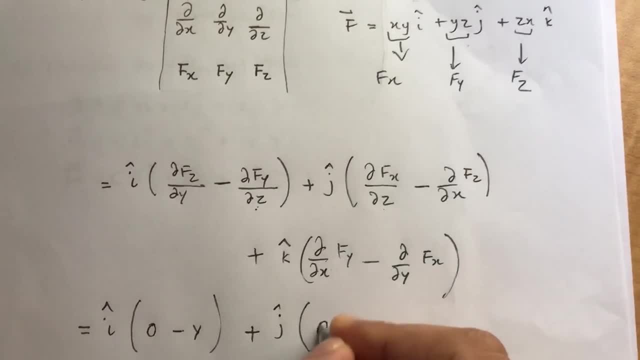 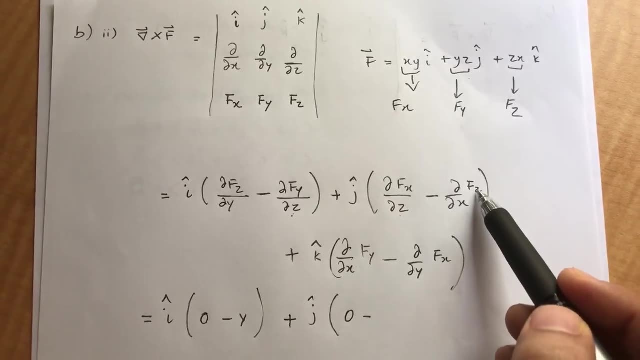 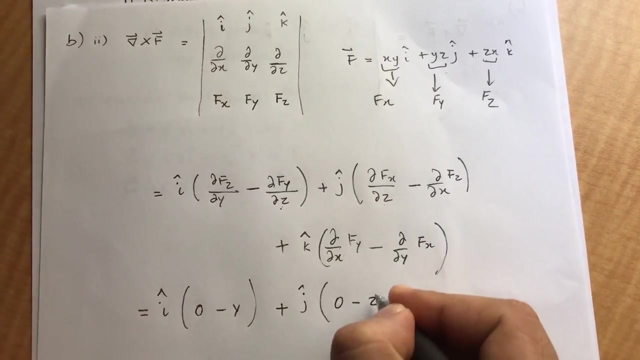 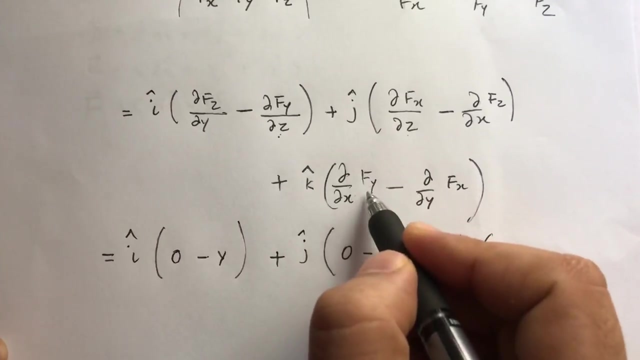 with respect to z, it's again 0, because I don't have z over there and then over here, if I actually take the partial derivative dF, partial derivative of Fc, with respect to x, it will give me z. finally, the third term over here, if I take partial derivative of Fy with respect to